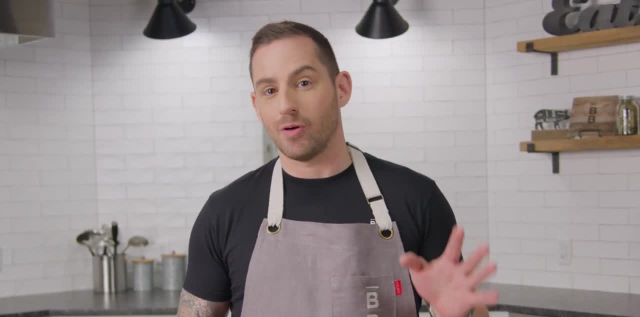 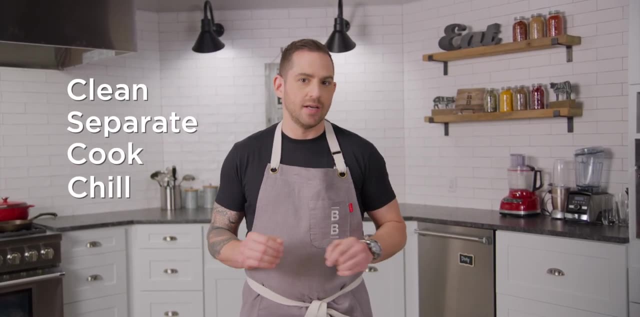 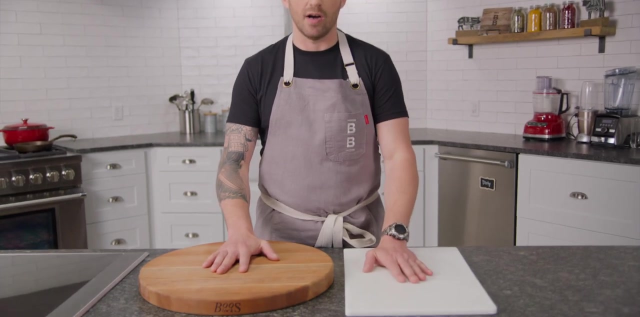 So, basically, the FDA has already done most of my work for me, and they break it into four processes. There's clean, separate, cook and chill. What do each of those things mean? All right, well, when it comes to cleaning, first and foremost, it comes down to the surfaces that you're working on. So 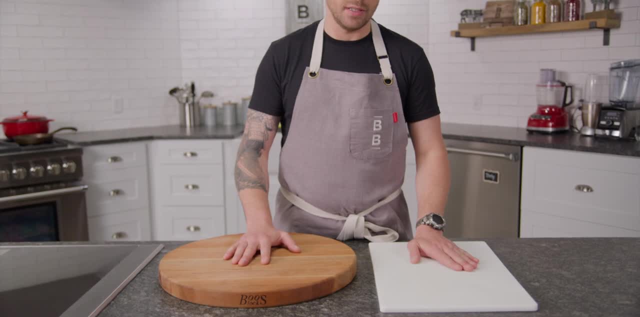 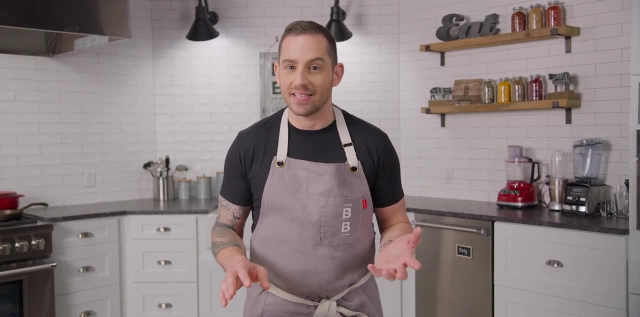 I've got a plastic cutting board that I use for raw proteins and then a nice cutting board that I use for everything else, If you don't have two separate cutting boards. basically, what you want to do is sanitize your cutting board in between every use, And even more. what I like to do is 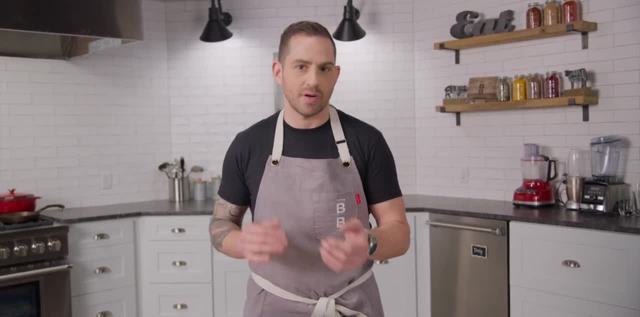 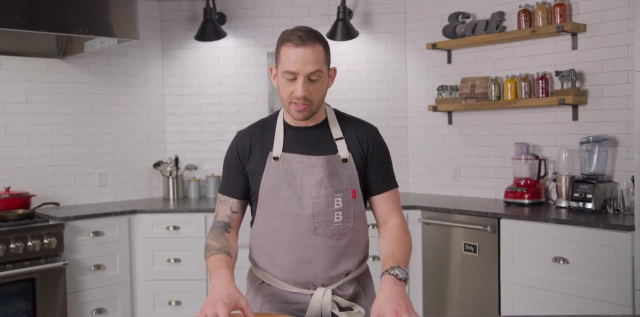 save my raw proteins to be the last thing that I cut on the board when I'm prepping a meal. Then I have no worries at all, and I will still wash and sanitize in between every use. Now, cleaning also means the surfaces around the area. 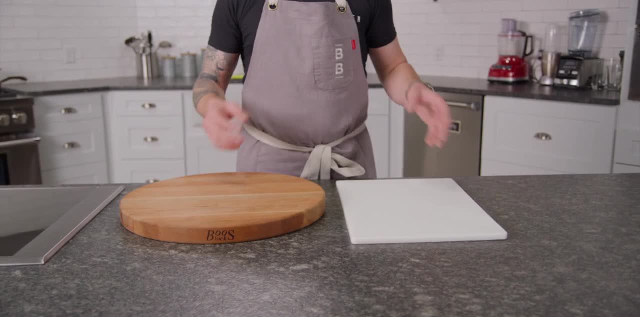 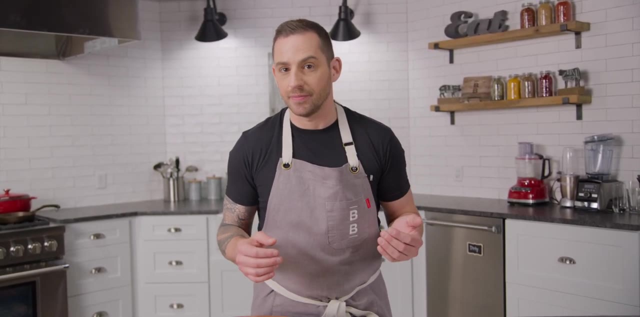 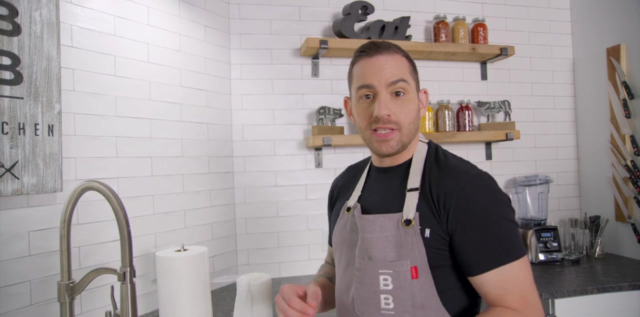 that you're working. So that means the countertops, It means drawer handles, It even means the sink itself, And I'll show you exactly what I do at the sink. For the sink itself, what I like to do is, once I'm done, washing up or in between, using raw protein and anything else. 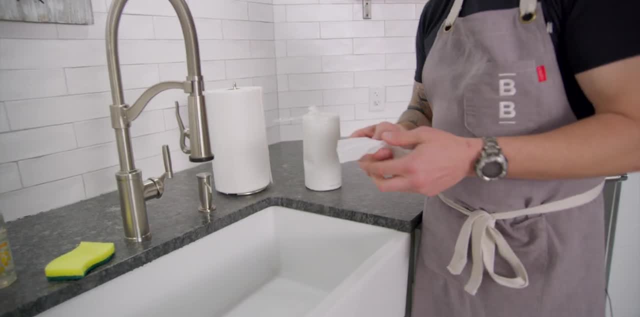 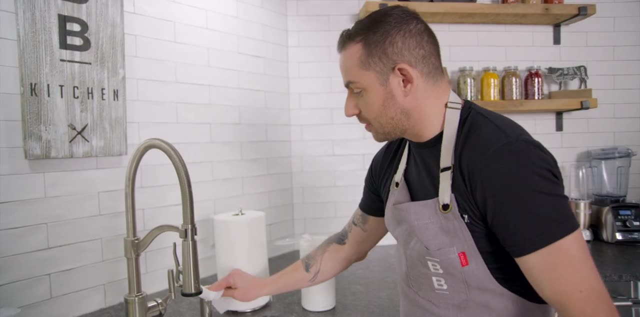 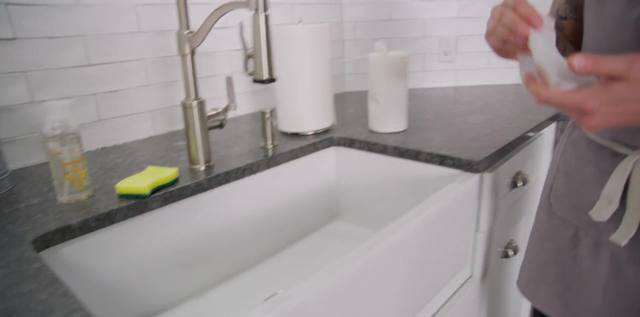 I'm going to sanitize every surface that I touched And I'm using a basic sanitary wipe And I'm going to wipe down the spigot. I'm going to wipe down the sink handle, the soap dispenser, even the inside of the sink. Give that all a good wipe, Make sure everything is nice and clean, And I'm 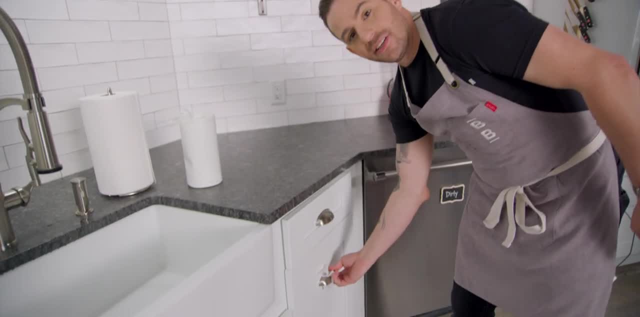 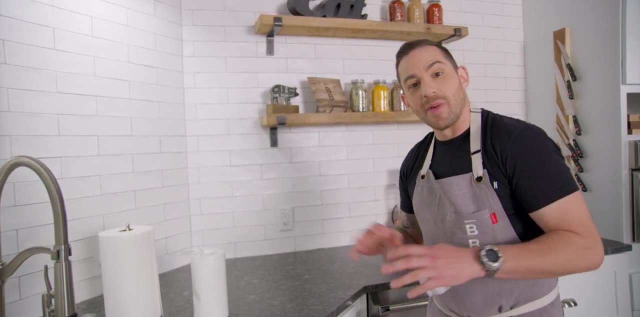 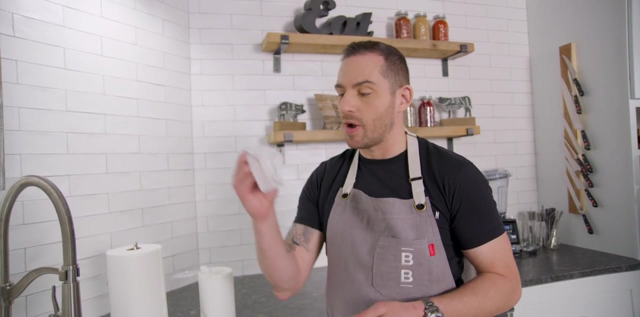 going to take it one step further and I'm going to make sure I get the handle to my trash can right underneath in there, Because, Lord knows, grimy fingers are getting in there. no matter what you do, As far as cleaning goes, every handle you touch, even the refrigerator door handles. I'll give them a wipe down. 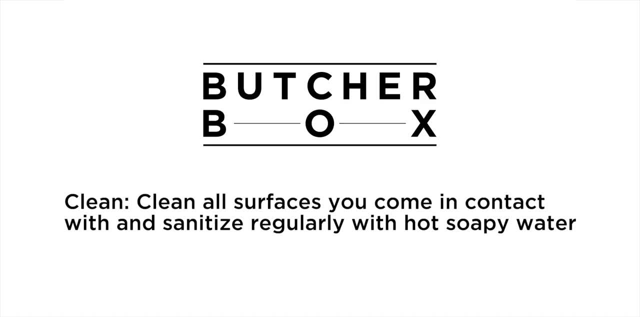 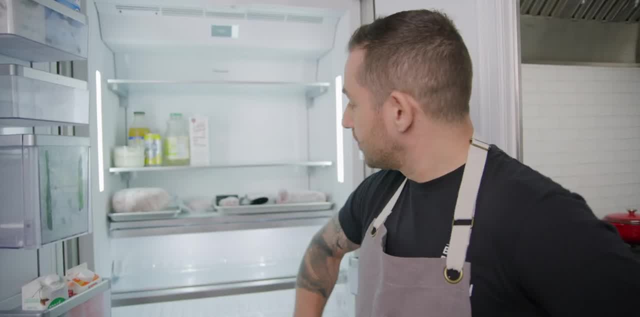 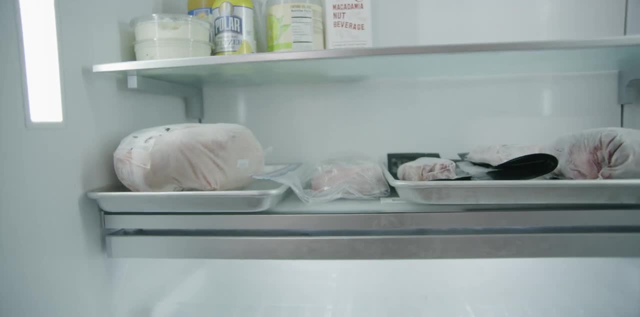 with a sanitary wipe in between my processes. Separate means starting with the refrigerator, keeping all of my protein separate while they defrost. So I've got chicken on a pan with a little bit of a lip. Now, of course, if you don't have room for pans, individual Ziploc. 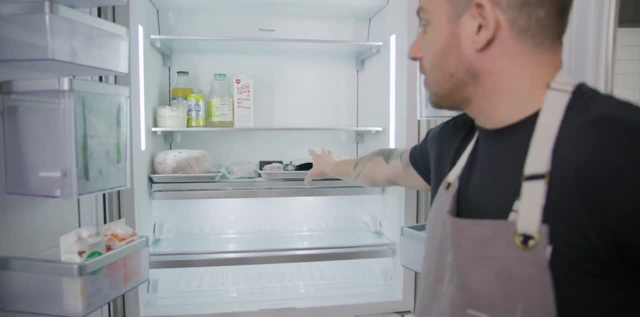 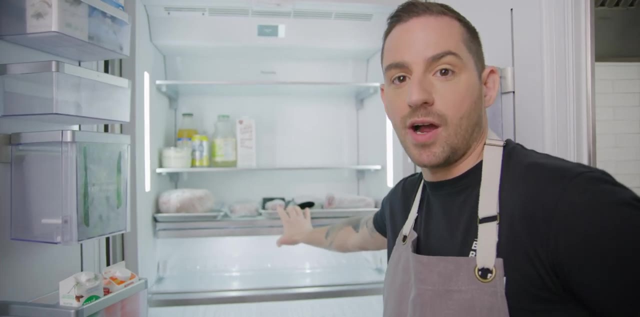 pans work really well And basically I want to make sure they're all separate. And then, even further, I make sure they're separate from other items in the refrigerator, So I put them on the lowest possible shelf to defrost and everything else will be above and separate. Now, separate can also mean using different cutting. 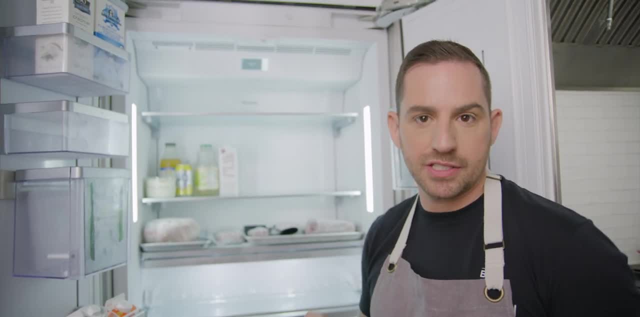 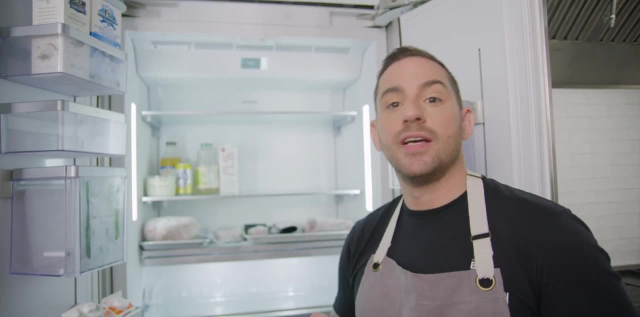 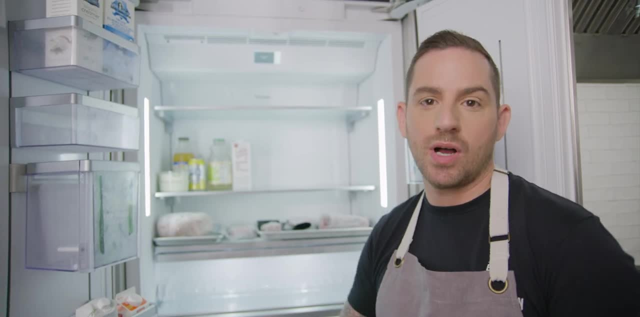 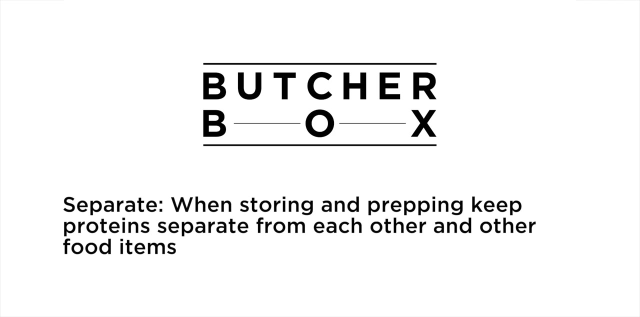 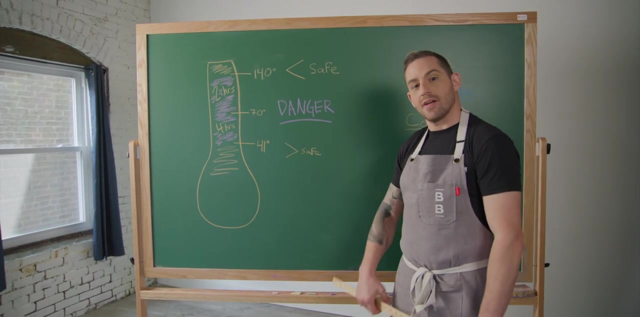 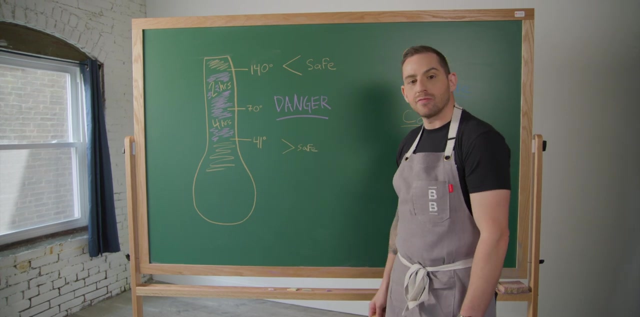 couple of different kinds of proteins going into one dish? Well, the answer to that comes when we cook. When it comes to cooking, our goal is to stay out of the danger zone. So the FDA defines the danger zone as being between above 41 degrees Fahrenheit and below 140 degrees Fahrenheit. Above 140, bacteria. 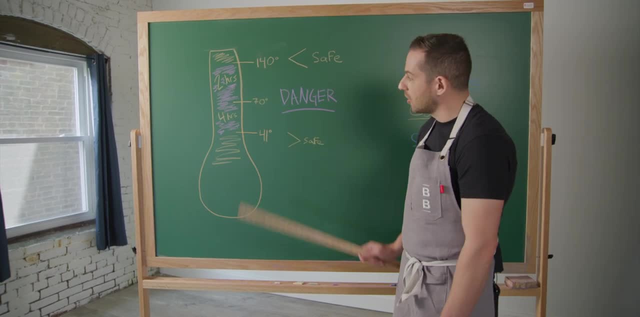 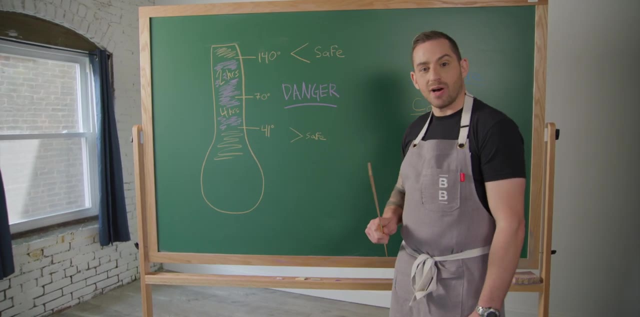 is dead Below 41,. it's inactive. Our goal is to get through the danger zone as quickly as possible when we're cooking and out of the danger zone as quickly as possible when we're chilling. Now, when it comes to actually cooking, 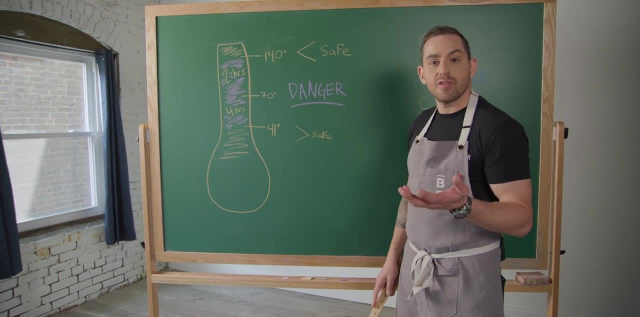 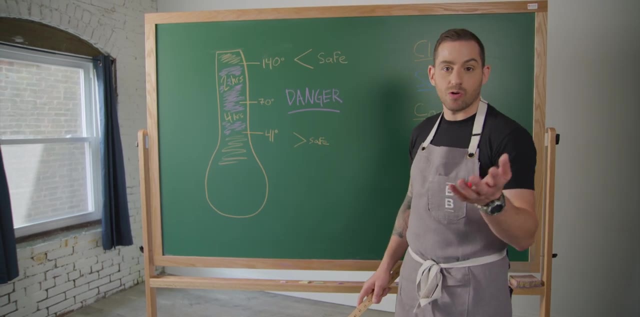 food. remember, with a steak it's the outside of the meat where bacteria can grow, And so a good hard sear takes care of that. That means you can comfortably cook a steak to rare or medium rare. When it comes to other proteins, you definitely 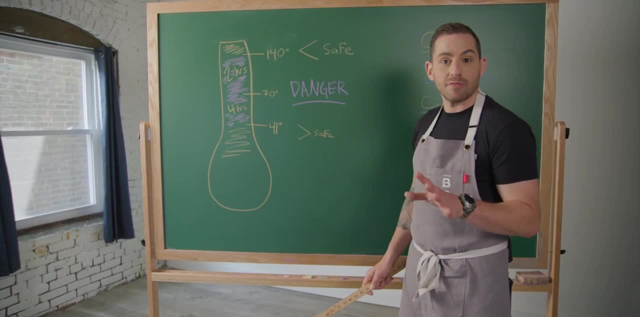 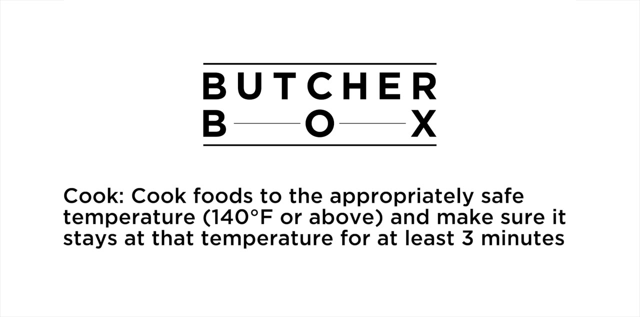 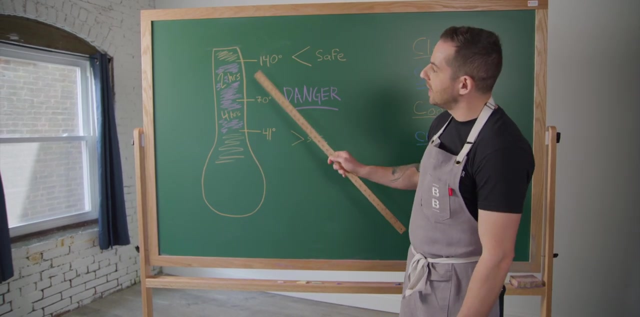 wanna cook it to 140 or above and let it rest there for at least three minutes. Now, when it comes to chilling food, same idea. we wanna get out of the danger zone as quickly as possible. FDA recommends a maximum of two hours. going from 140 to 70 degrees and a maximum of four hours from 70 to 41. What that means for you is, as soon as your food has cooled down a little bit, pop it in the fridge and that will take care of the rest. So that's really what it comes down to. Now, if you're wondering about immersion circulators, that sort of thing where you're cooking at a lower temperature, well the answer: there is time. Bacteria will actually die, but it takes longer. 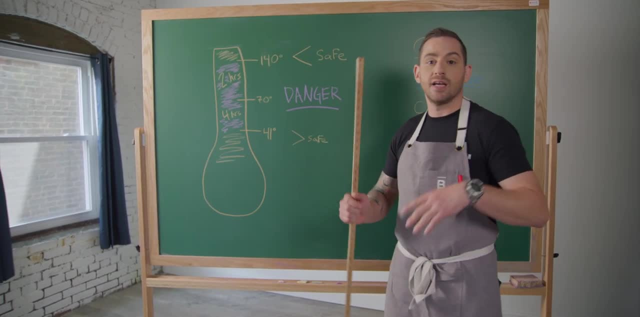 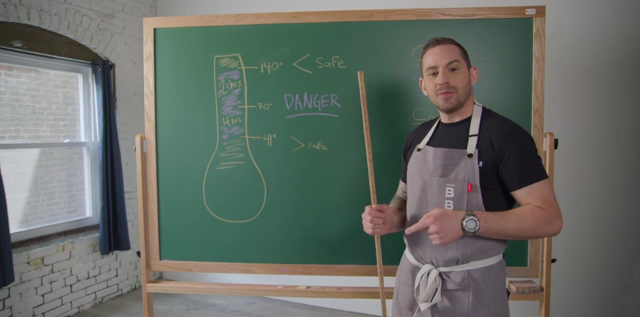 So make sure that you do a little bit of research before you start cooking steaks in an immersion circulator at 130 degrees, And if you're cooking them at 140 degrees or below. Well, I hope that clears some things up for you. I'm Yankel, go be safe out there.